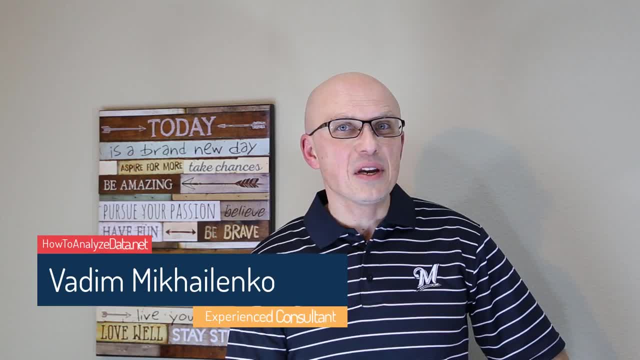 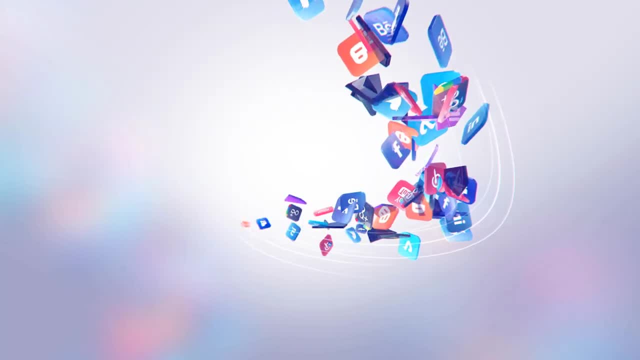 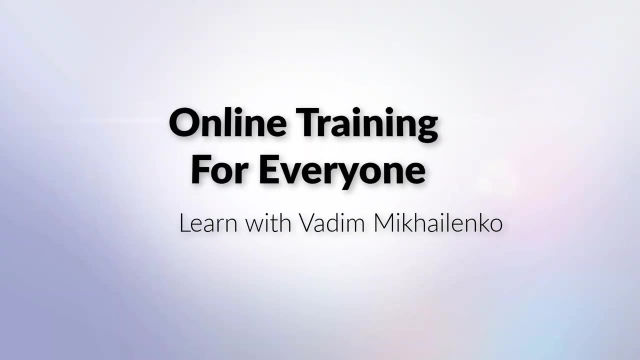 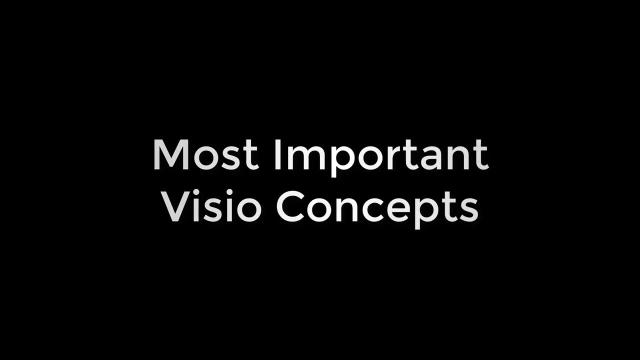 Hi there, my name is Vadim Mikhalenko, and in this quick video we're gonna look at how you can create flowchart diagram in Microsoft Visio, Coming up an online training for everyone. First, let's overview three most important Visio concepts: Shapes, stencils. 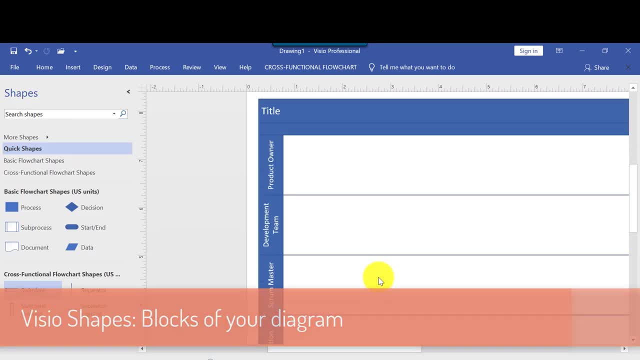 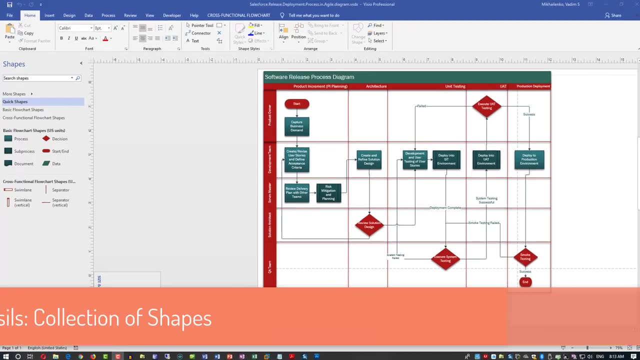 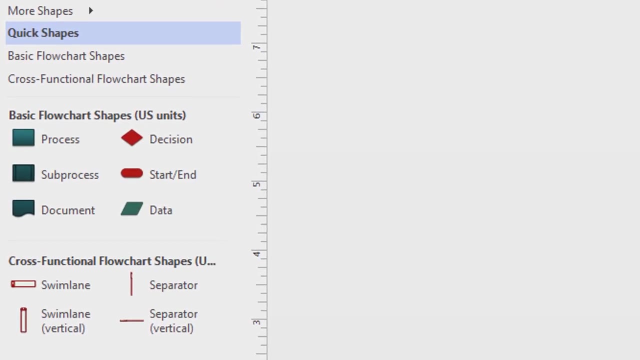 and templates. Visio shapes are objects that you drag onto your drawing page and this is what you use to build your diagram. Visio stencils is a collection of shapes. Shapes in each stencils have something in common: They follow the 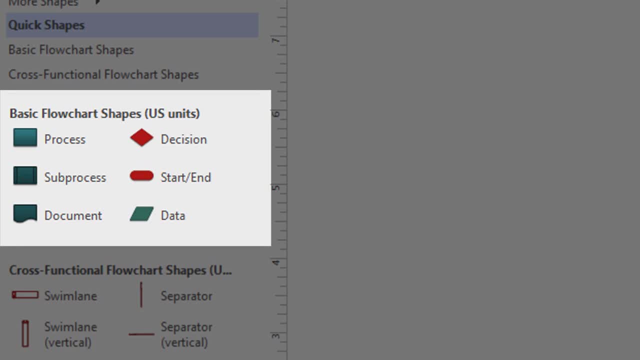 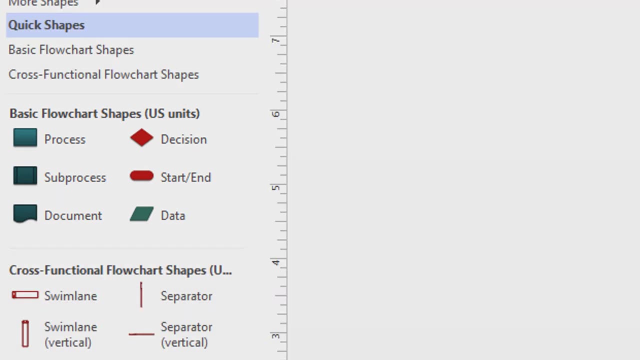 similar pattern and similar theme. For example, basic flowchart stencil has process, subprocess, document, decision, start and end and data shapes, And cross-functional flowchart has swimlane separator, swimlane vertical and separator vertical shapes And templates used to create particular kind of diagrams When you want to create a 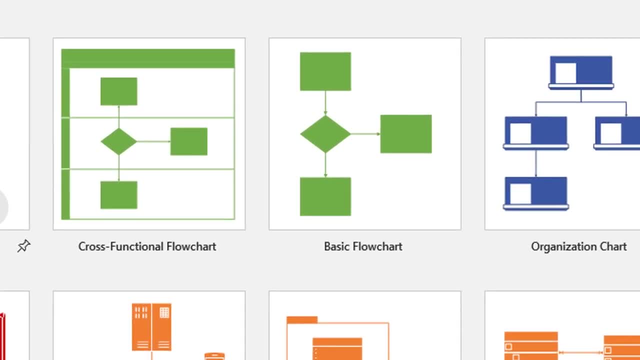 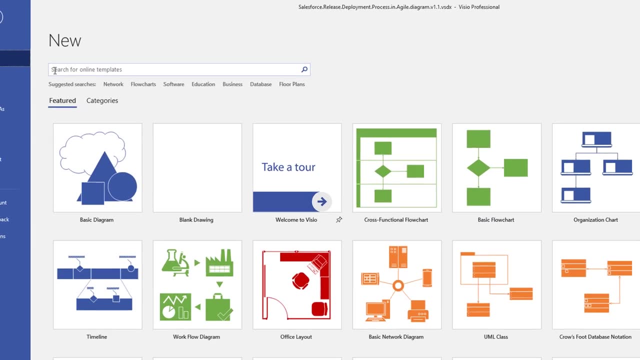 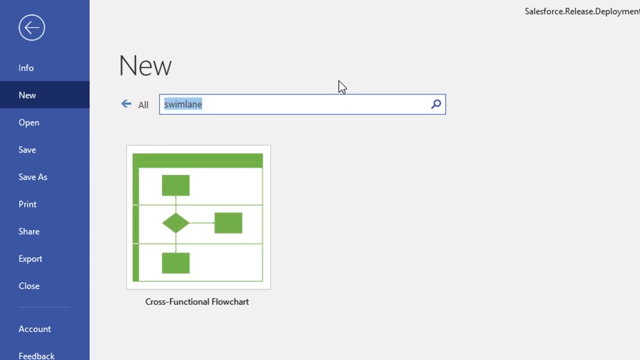 diagram. start with the template for that type of diagram, which you can search when you start new Visio diagram, For example, to create a new cross-functional flowchart diagram, navigate to file tab, click on the new type in swimlane and then select cross-functional flowchart. 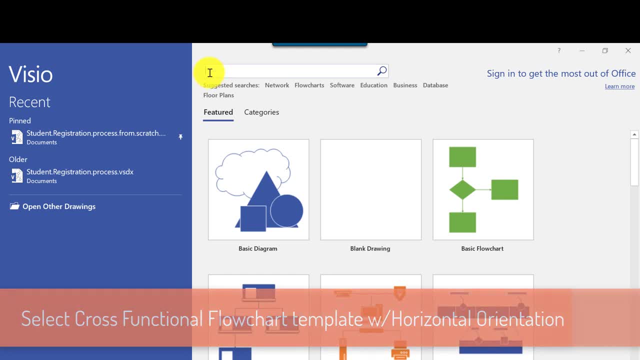 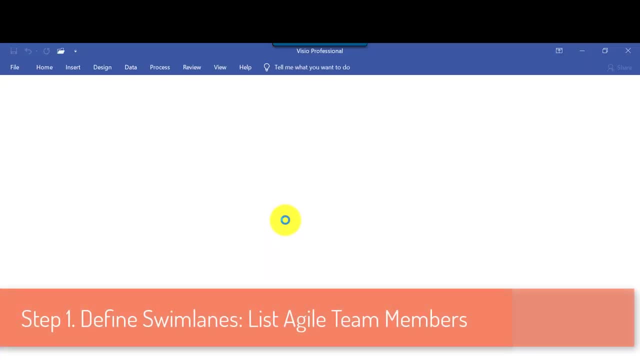 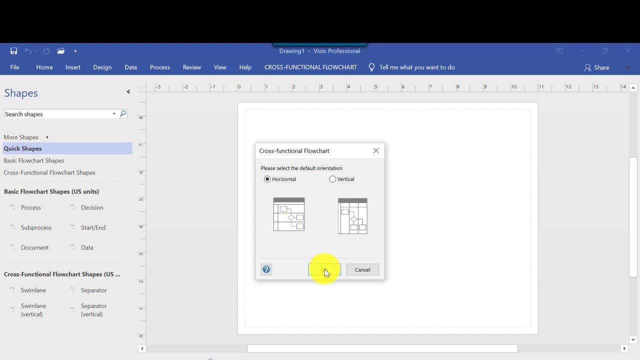 diagram. Now let's go ahead and create a simple flowchart diagram. To do that, navigate to the new tab and type flowchart in the search bar and select cross-functional flowchart diagram. Next, select the horizontal type of the diagram, because this fits the best to what we're trying to accomplish. Visio. 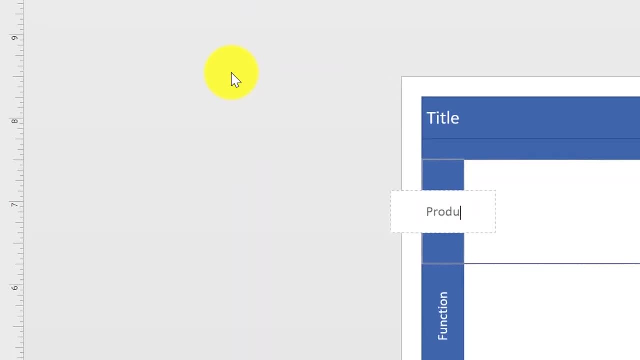 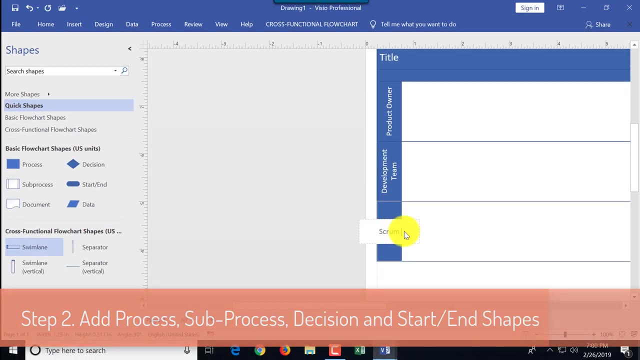 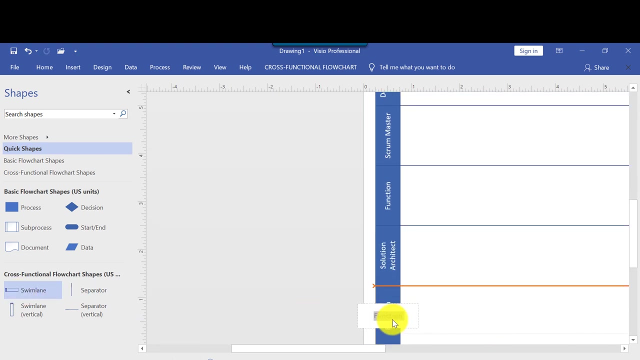 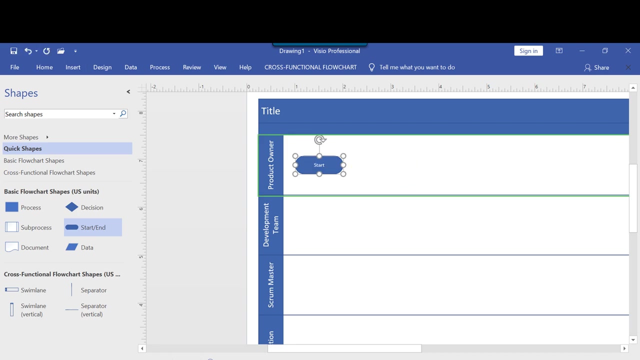 created the template with the new swimlanes, Since we are defining the deployment process, need to identify agile team members for each swim lane and type their names. you do this by clicking on the swim lane title and typing the role of the team member. next you start dragging and dropping shapes from the stencil for 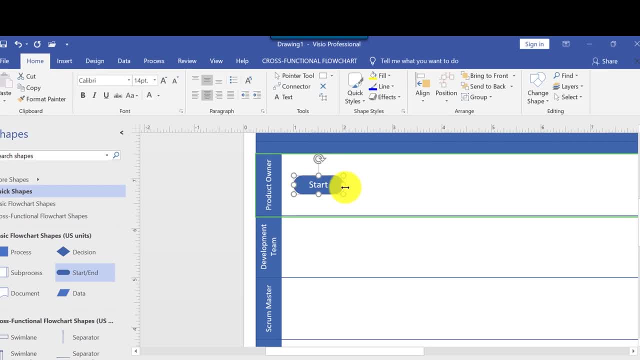 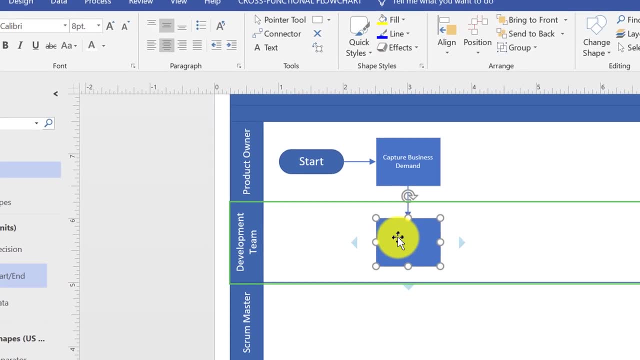 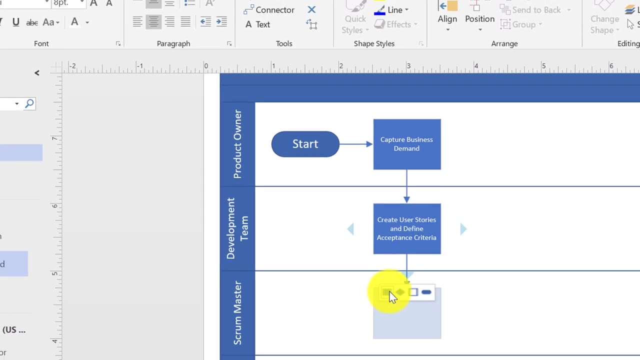 basic flow chart diagram into the diagram itself and then you connect those shapes based on the functions that you're trying to describe. you start with the start shape and then add process shapes and then connect them in the right sequence. that would describe what each team member will be doing for. 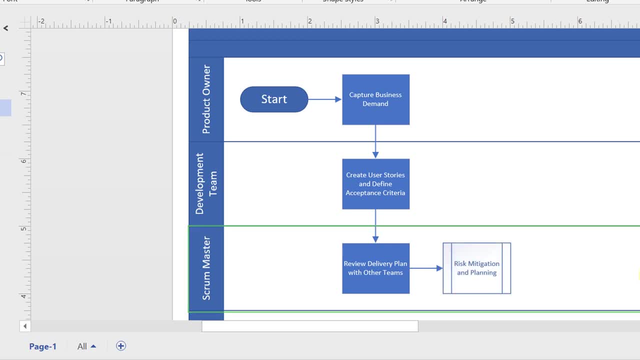 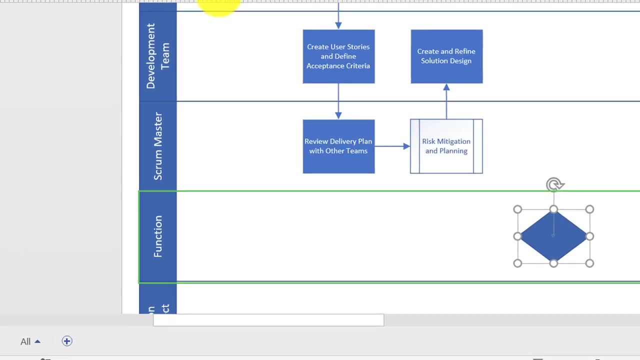 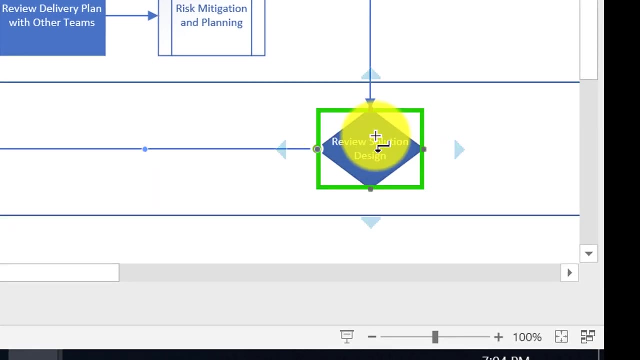 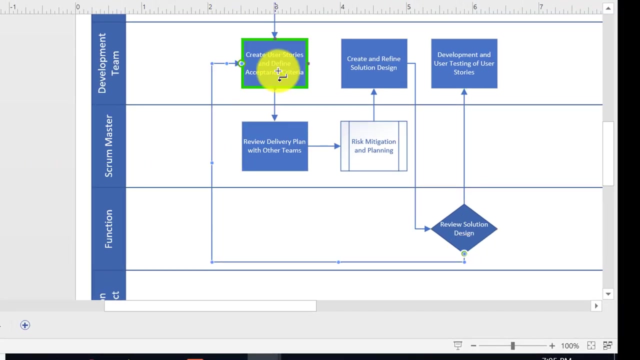 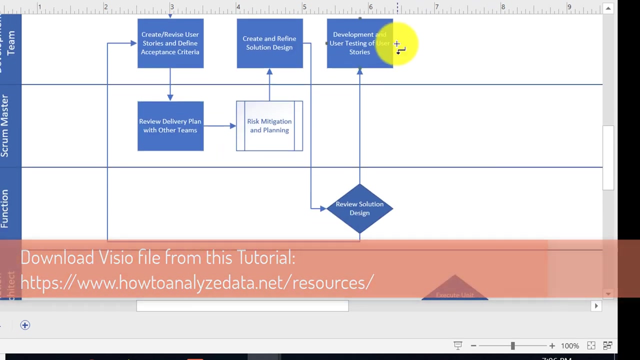 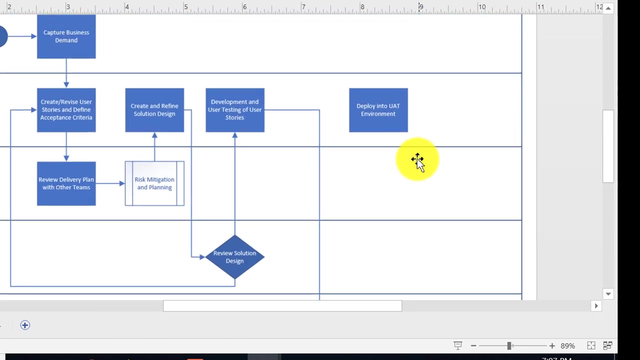 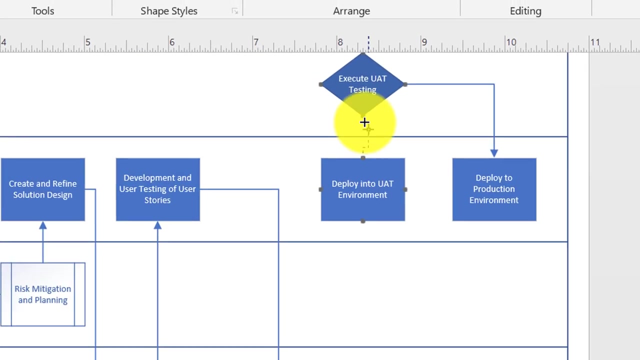 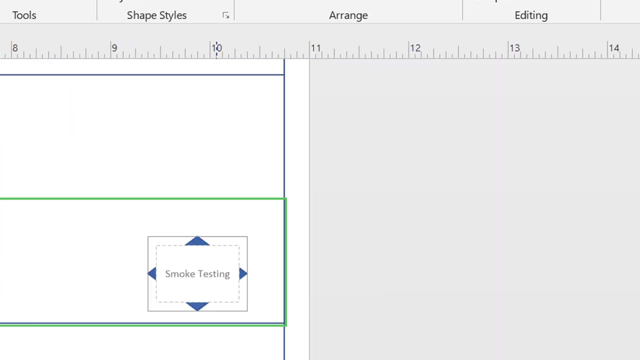 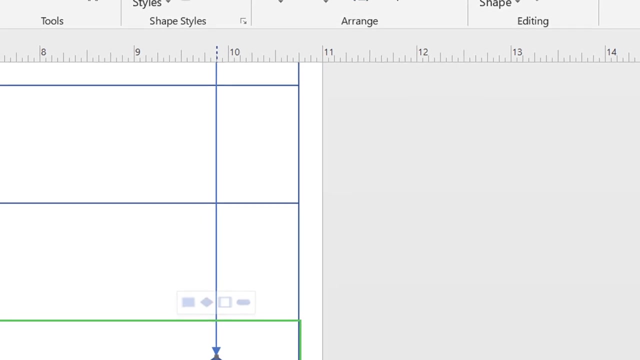 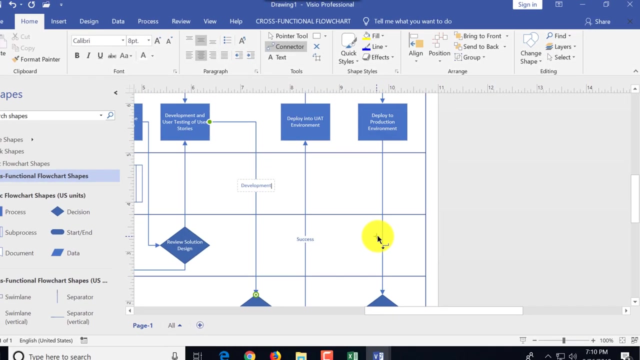 optional steps use sub process and for decision steps, you use decision shape. if you would like to follow along, feel free to download the template for this diagram from www. how to analyze data. dotnet slash resources GUI. yes, yes, once diagram is finalized and anyununsa type functions, now Perov's course 지금. 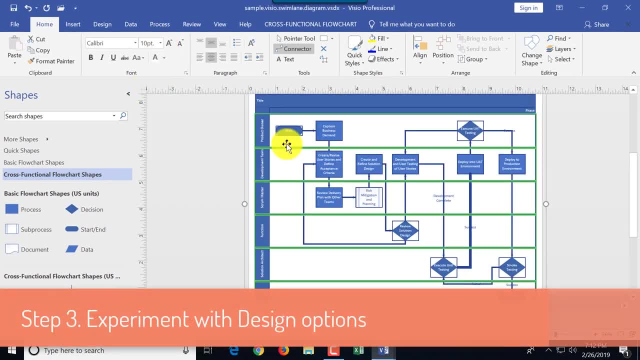 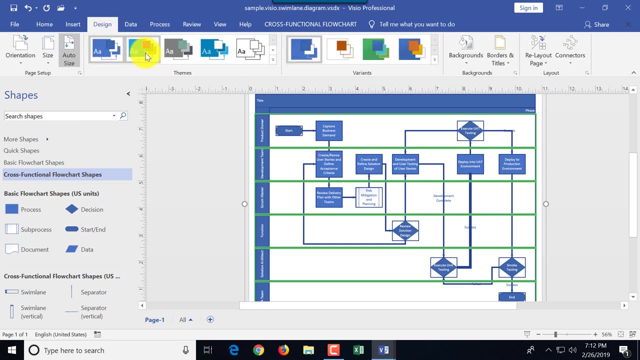 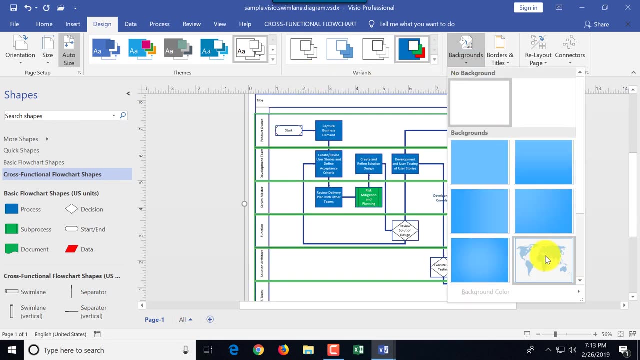 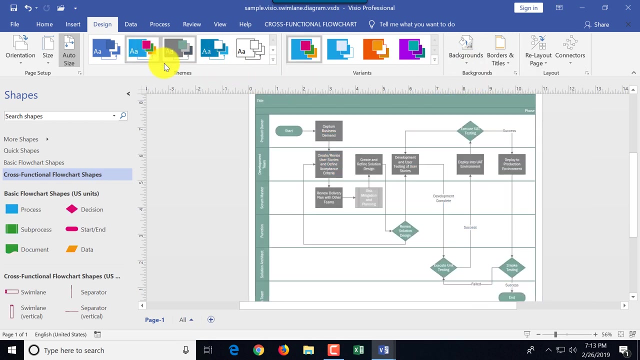 complete. you can experiment with the different design options. If you go to design tab, you have a lot of choices in terms of design themes, variants and backgrounds. Each theme has its own set of variants and you can pick any background that you'd like, Because software deployment 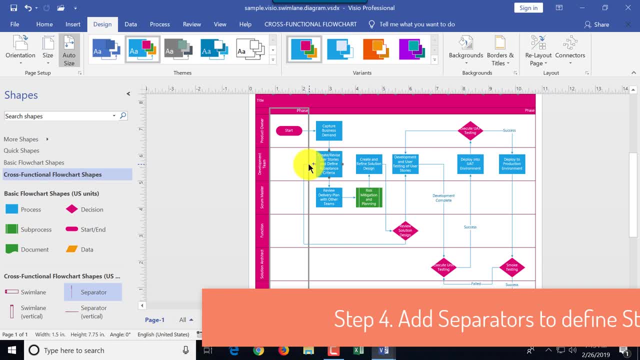 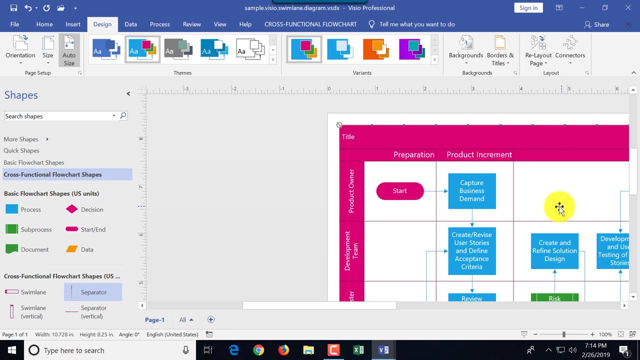 process is very sequential. you can define different stages for the deployment process. For example, key stages for release process are product increment, which is PI planning, architecture, unit testing, management and development. If you want to see the process in more detail, you can click on the link in the description.